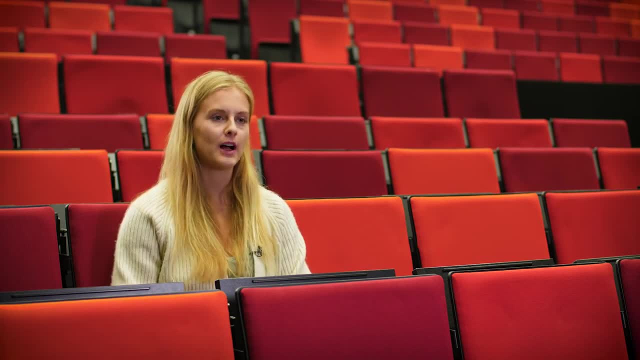 your relevant documents to the FHAS admission portal. After a while, you'll be contacted by a member of the staff for an interview. They want to hear more about your motivations for studying this degree And then, after a time, they will contact you to let you know whether or not. 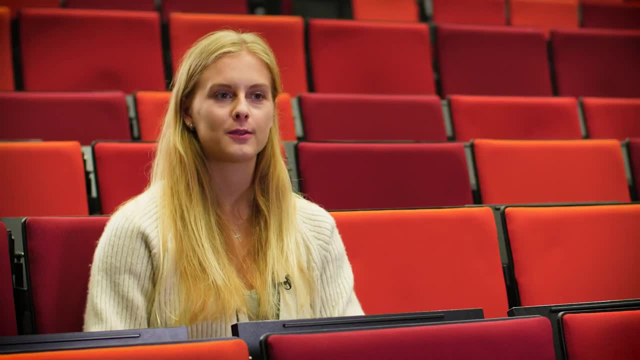 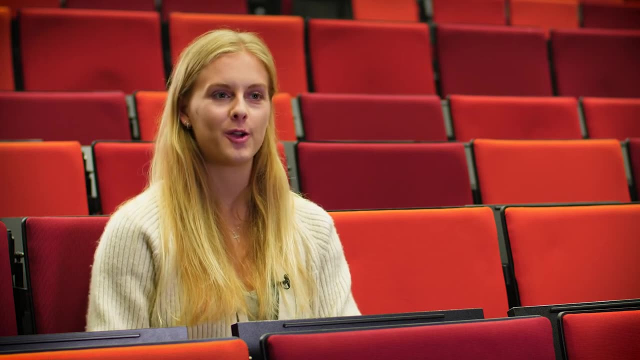 you've been accepted to the program. So the master's degree is a full time program, but luckily they have arranged the courses in a way that it makes it quite easy to still hold a part-time job. I know myself and most all of my classmates all work aside from our degree as well. 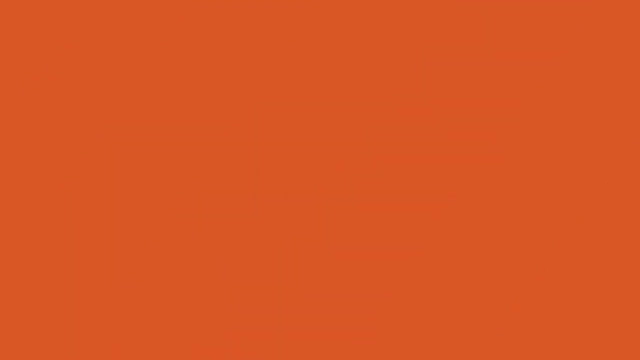 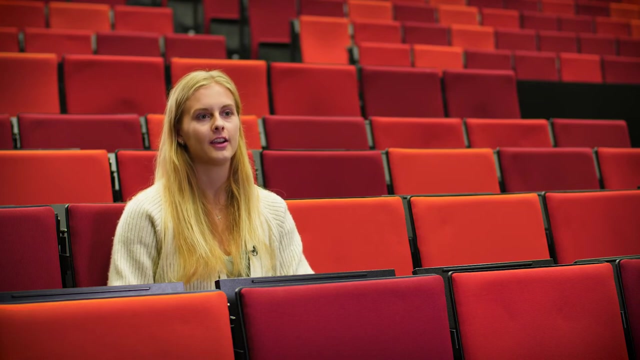 So it is still possible to manage your time effectively. The focus of this degree is really special because it's a really good mix of theory and practical subjects And there is a strong mix of subjects that you have to attend, But luckily there are also a number of electives you can take in order to specialise or deepen your focus in. 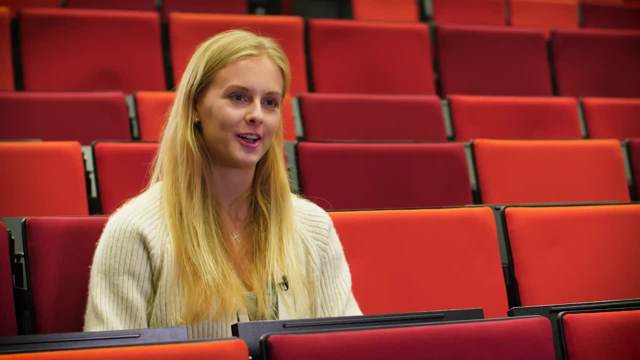 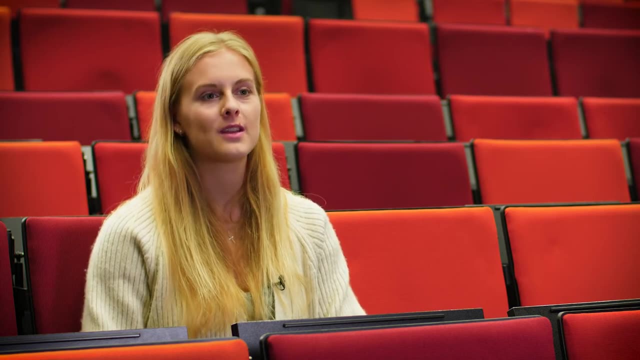 something that you are more interested in. So I think the lecturers here are incredible. they're so knowledgeable, so passionate about what they do. there's a really good mix of those who are academically focused, and then we have a lot of people who are in industry as well, with 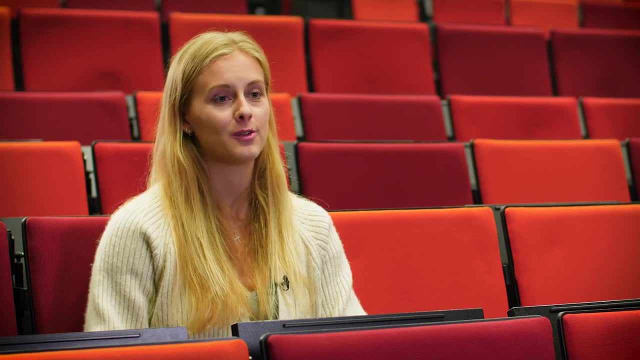 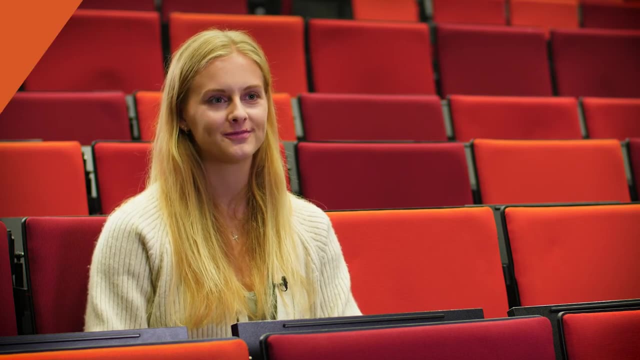 real experience in the real world and our lecturers are really personal. they know us by name, they're very friendly and I have a really good relationship with all of them. I think they're really good staff here. So the great thing about this degree is it prepares you to go into either. 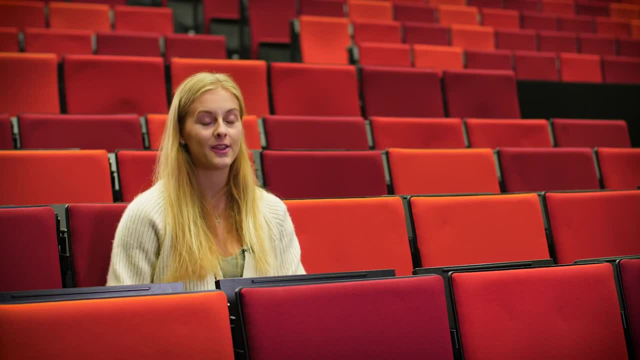 industry or into academics, depending on which one you prefer. and the great thing about HCI is it's such a broad field. you can choose your specialisation based on what you enjoy most. So people either become UX designers, experienced engineers or HCI consultants. Personally, I'm 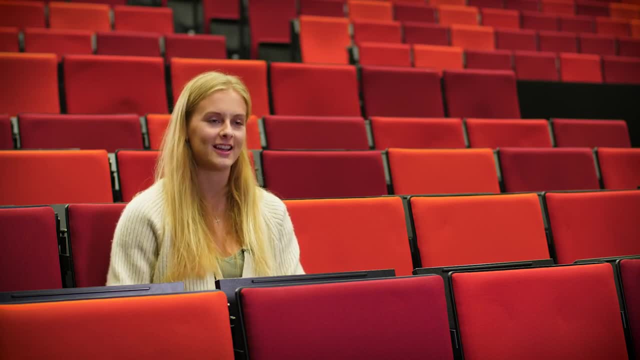 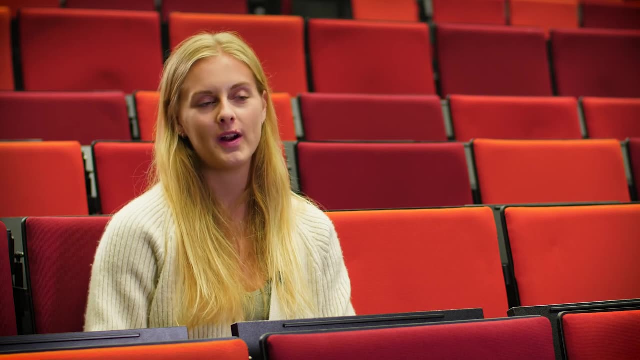 really interested in hybrid human AI creativity, so I'm going to take that into industry and see where I can go with it. I think the most unique thing about this degree is that it takes place at two different universities. So on the one hand, you have the FH Salzburg, which is very new and modern and has amazing facilities. 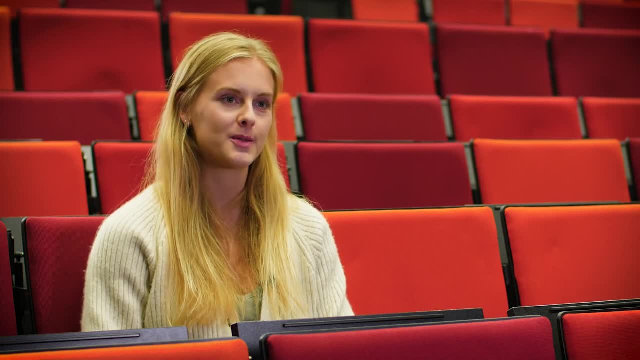 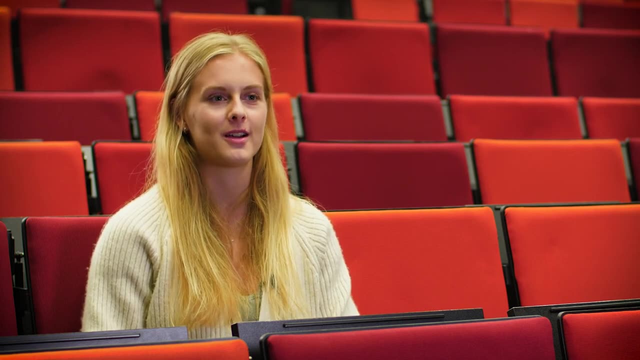 for learning more about technology. On the other hand, you have the University of Salzburg, which is older and more established and has great history behind it. So the mix of these two experiences, I think, is a very special part of this master's.